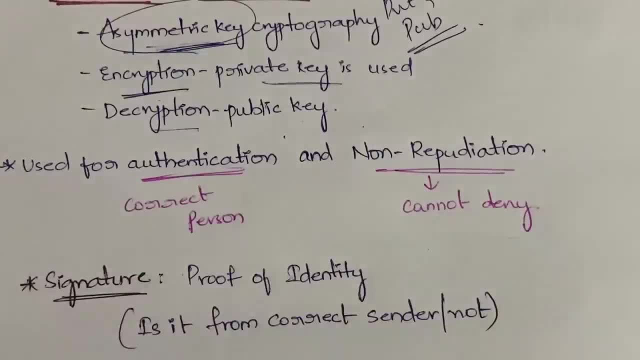 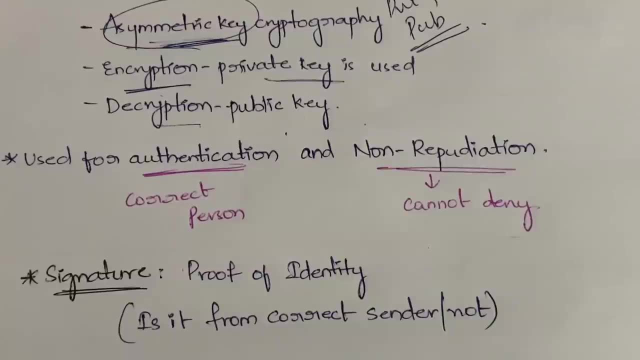 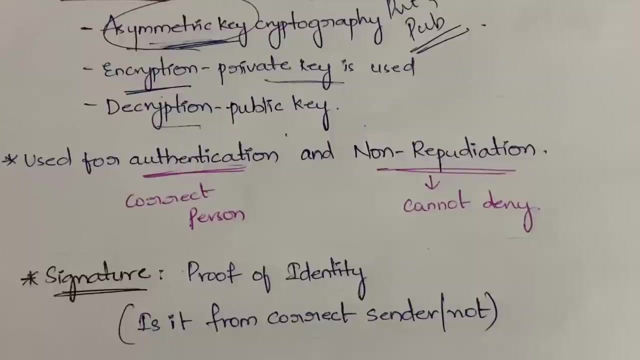 this is used for both authentication and non repetition. That is, like you know, the CR triad right: we have confidentiality, we have integrity, we have availability. Apart from them, we also have some concepts like authentication, non repetition. So what do you mean by authentication? is you are sending the message to the correct person or not? whether you're, if you want to send a message to your friend, So whether the message is being sent to your friend or not, your friend or to anybody else, So it ensures 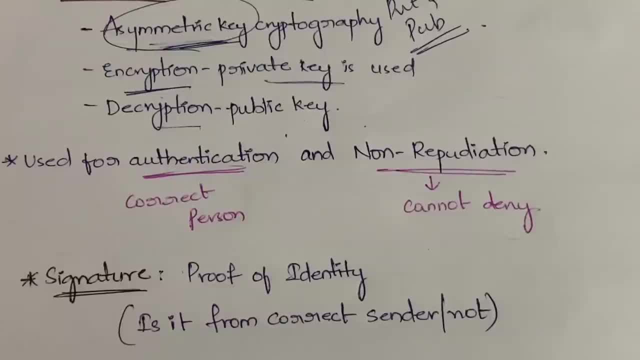 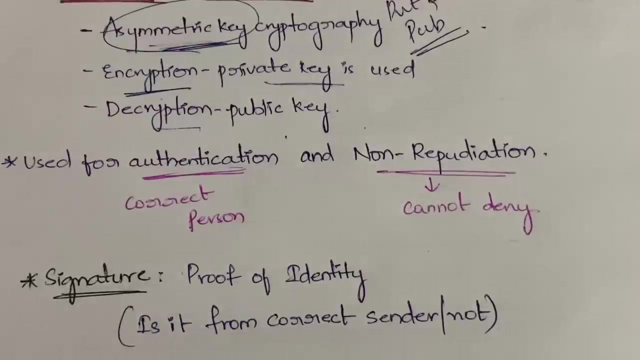 authentication that it is. it will be sending the message to the correct person, So the intended person to whom you want to send. to that person only message will be sent. Okay, this is what authentication. and next, what do you have? you have non repudiation. So what do you mean by non repudiation? it is very simple: you cannot deny the message of somebody's are telling you something. If I've sent you a message like hi, then you cannot deny my message. you cannot say that I did not get the message, So non. 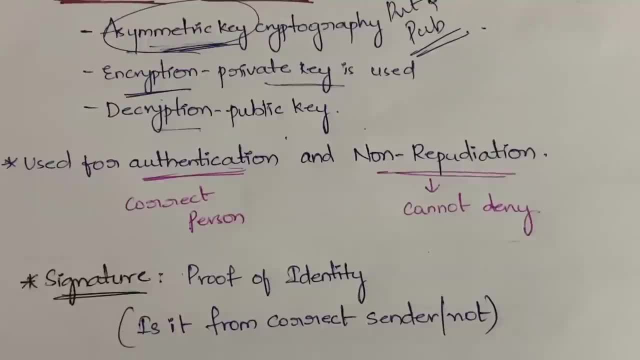 repudiation. that is uh, in some cases, what do we do in order to skip the work or, you know, in order to escape? so we will be like i do not get the mail or i did not get the message. we'll be doing that right. so here, that will not work right. and first of all, before moving into what digital signature? 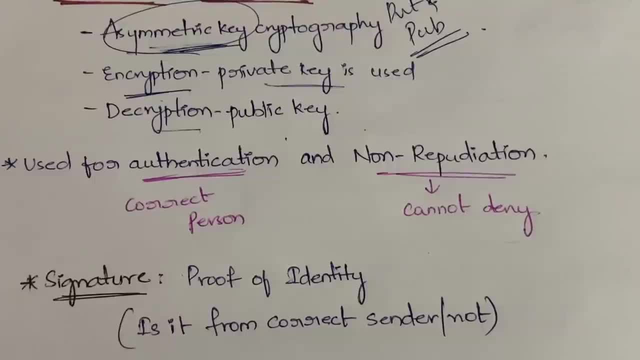 is. you know what a signature is right, why you have to sign each and every. when you apply for your other card, when you apply for your passport, when you apply for your- uh, whatever it is- pan card, whatever it is, they'll be asking you to sign. when you sell a property, when you buy a, 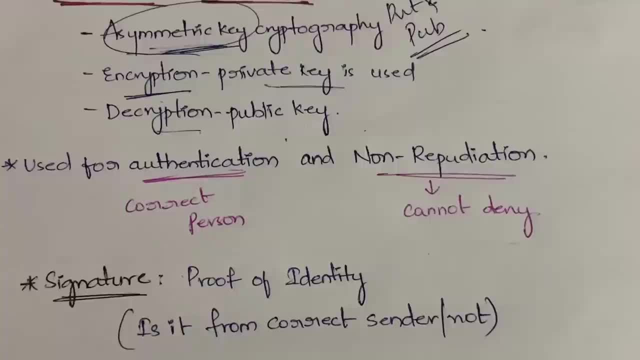 property bank account everywhere for all the transactions and all. why? because it is a identity got it. if you are signing, then they will be checking your signature against the signature they have in the database and if it is matching then they'll allow you to do a transaction right. 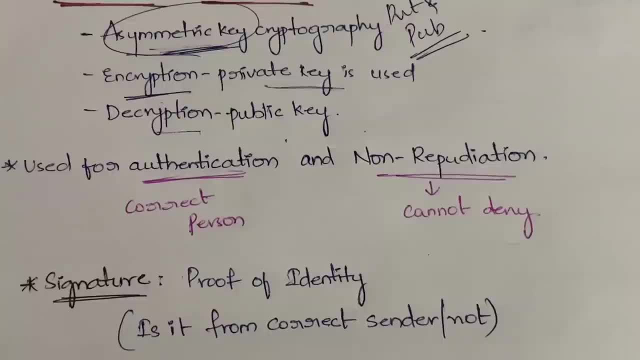 so it is a proof of identity, whether it will check whether the message is from the correct sender or not. in case of, in the terms of network security, if you're speaking, it will check whether the message is coming from the correct user or not. got it done? so this is about the signature. now let us understand how digital signature will work. 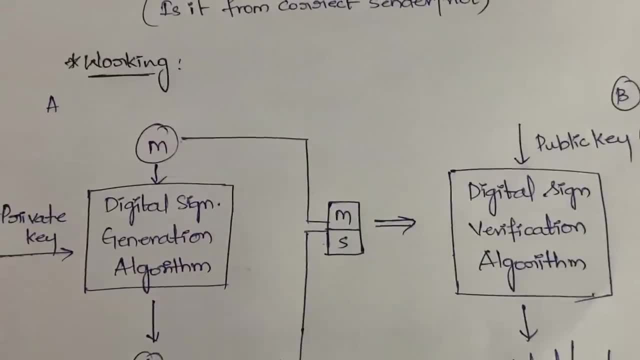 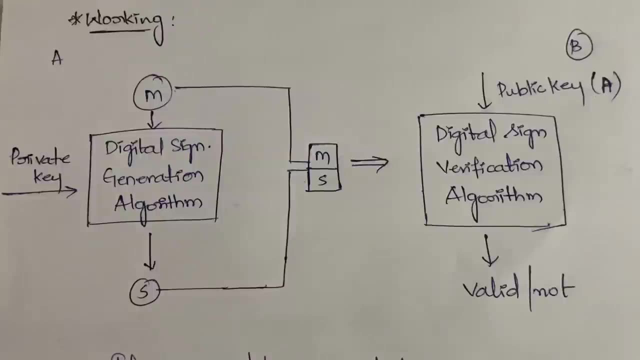 got it. so this is the diagram which is showing you the working of digital signature algorithm. very simple, don't? um, you don't get confused. first what happens is you will have a digital signature generation algorithm. okay, so first what happens is you will be taking the private key. this 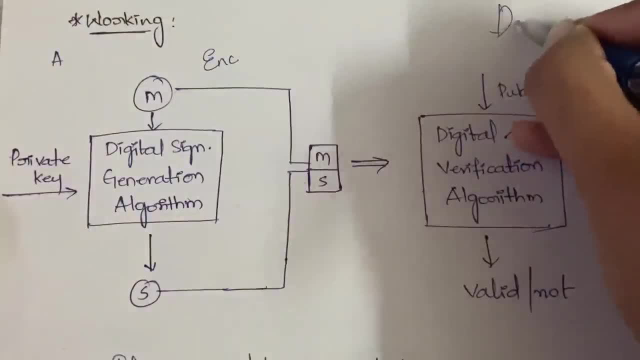 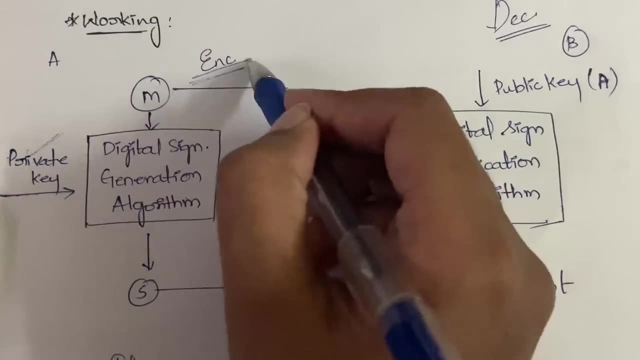 is the encryption end right? this is the encryption end and this is the private key and this is the decryption end. at the encryption end, which key? we are using private key. as i said you in the beginning of the video itself, at the encryption end we will be using the private key and at the decryption end, 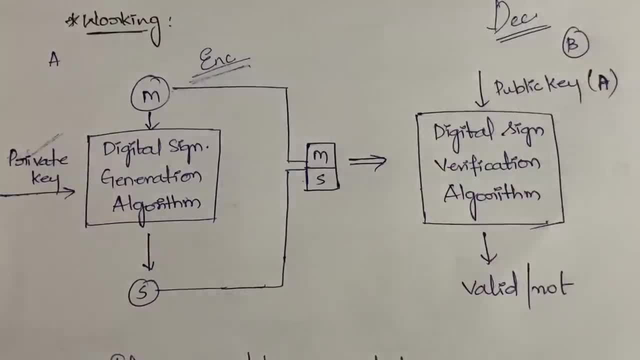 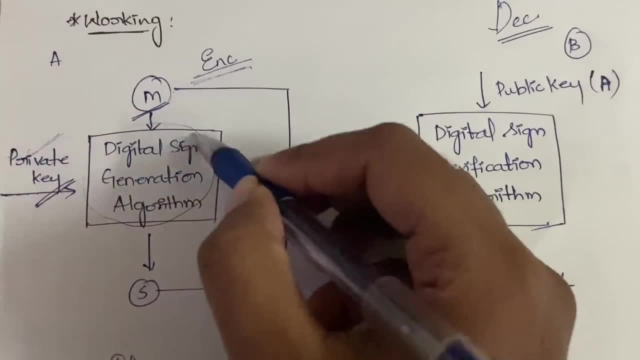 we will be using the public key right now, here, first. what will happen is you will be giving the message and the private key as an input to the digital signature generation algorithm. got it so? based on the message and the private key which you have given, a signature will be generated from the. 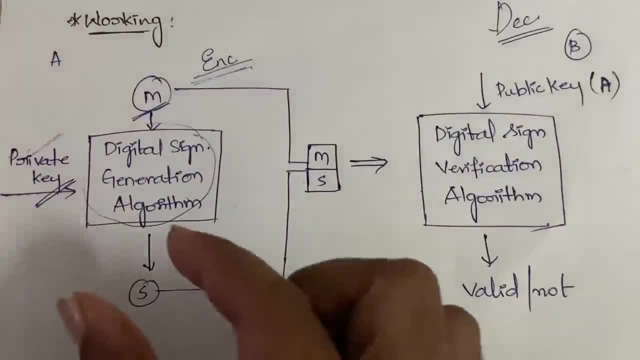 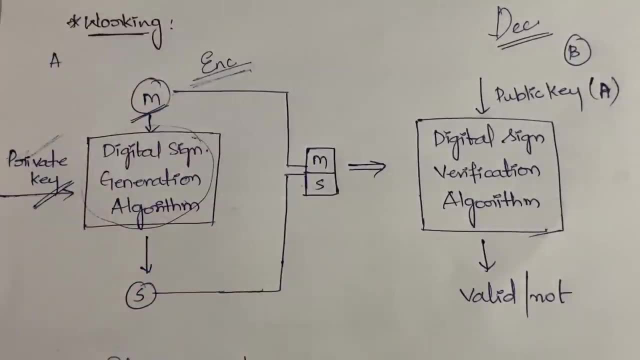 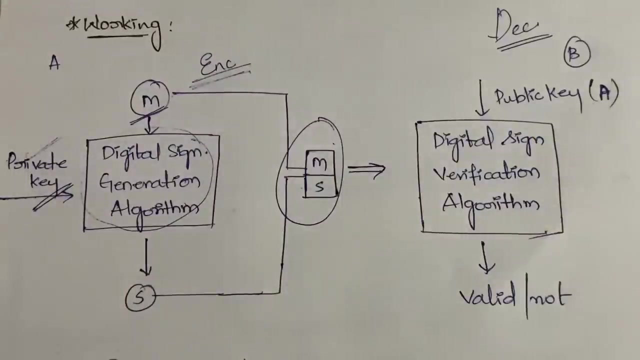 digital signature generation algorithm got it. so once the signature is generated, now this message and signature, both are combined together- see message and signature. both are combined together and here, and it is sent to the receiver. both are combined together into a single message and that single message is sent to the receiver. now what receiver will do? as usual he'll be doing. 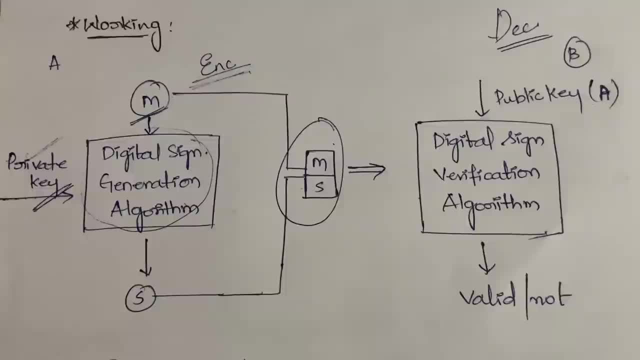 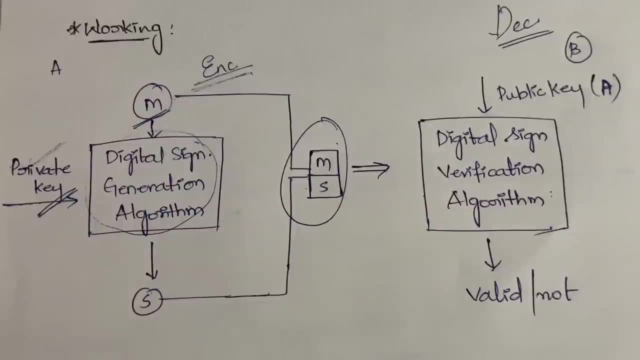 the decryption process. right now how he will do the decryption process, he will be using the public ko a got it private key of a who will have a itself will have because it is private- private in the sense only i can have, only i can access to that, only you can access to that. you cannot share it. 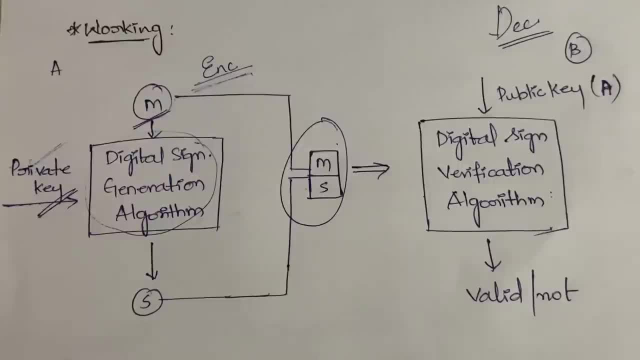 it is not public. you cannot even share it with your friend. got it here. public key of a. why? because you are using the private key of a got it. so, since you are using the private key of a, you need to use the public key of a at the decryption end right now. here what he. what happens is the receiver. 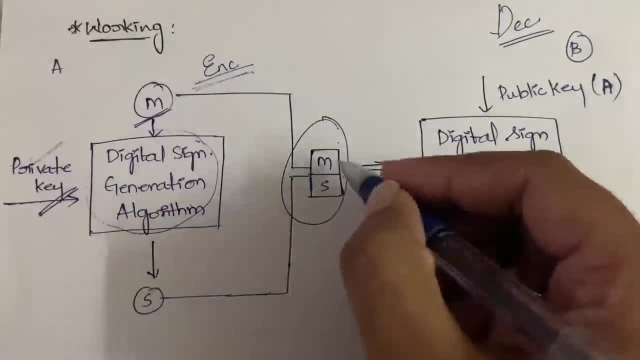 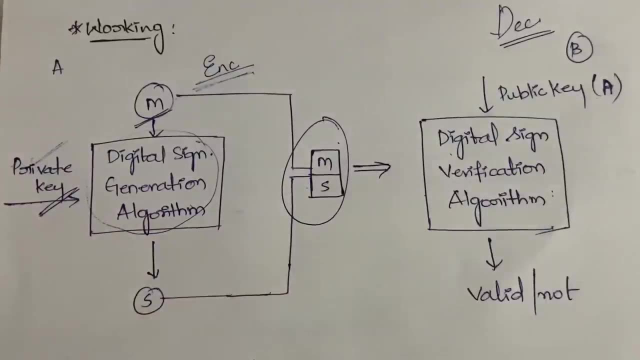 will be using the public key of a and the combined message and he will verify this with the. you know, with the help of digital signature verification algorithm. got it and what will be the output of this algorithm? it will say whether it is valid or not. how it will say whether it is valid or not. 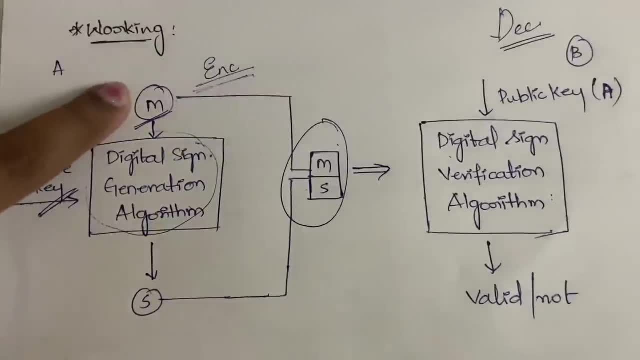 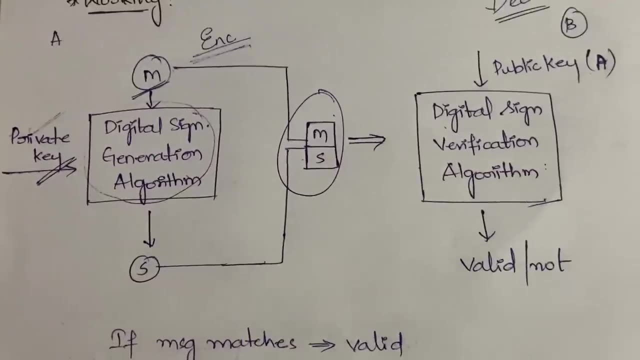 if the message is matching with the initial message which is being sent from here, then it is valid. if the message is not matching, it is not valid, got it? so here we have two algorithms: digital signature generation algorithm, digital signature verification algorithm. in generation algorithm. what are the? 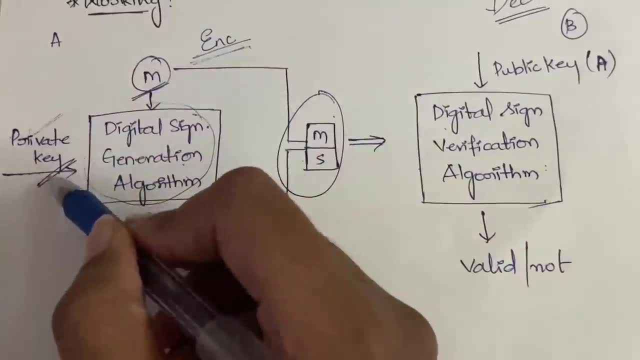 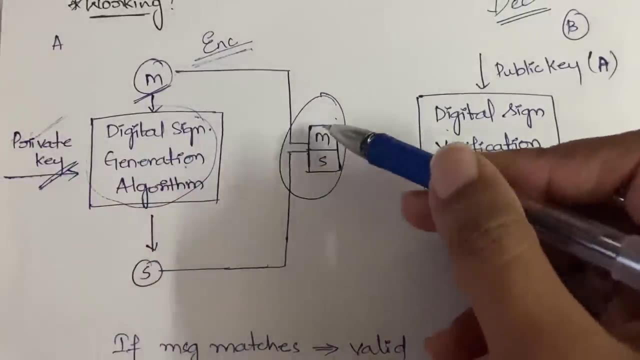 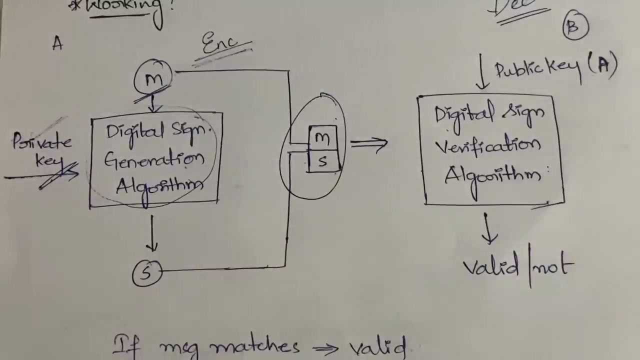 inputs: the plain message, the plain text and the private key. right now, here for digital verification, what? what is the input? the combination of message and signature plus public key. this is not at all complicated, just related to the encryption and decryption process. in encryption, decryption process, what is happening? we will be giving the ciphertext ciphertext, sorry, plaintext, plaintext. 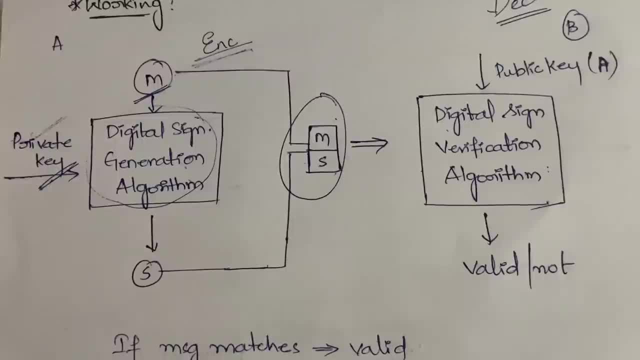 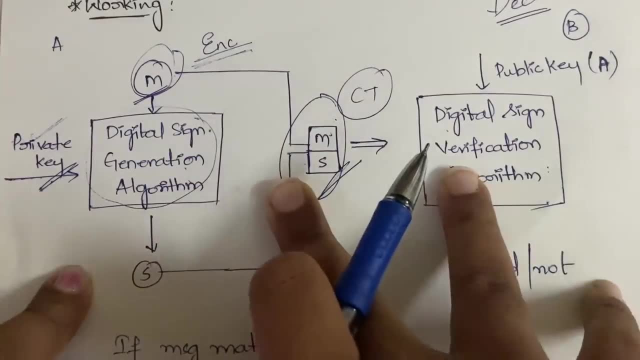 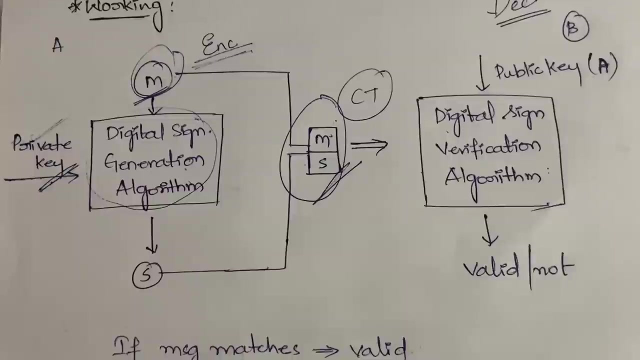 is converted to ciphertext. again ciphertext back to plaintext, right? so the same happens here. so here the plaintext is m and as a result the ciphertext assume ciphertext. is this combo right? and the ciphertext is checked, it is a plaintext is obtained. so here, normally in decryption what happened? we will be directly getting the ciphertext. we will not check the ciphertext with anything. 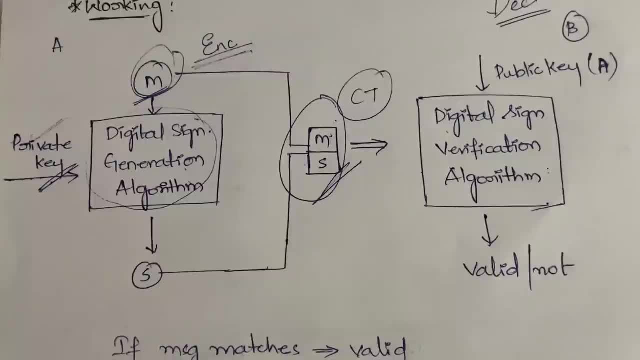 right, but here we are checking the ciphertext, the plaintext which we have obtained with the original message. if it is matched, then it is valid. if it is not matching the signature is not valid that we have somebody the signature, maybe the strokes are in some cases. you know, I have my I. 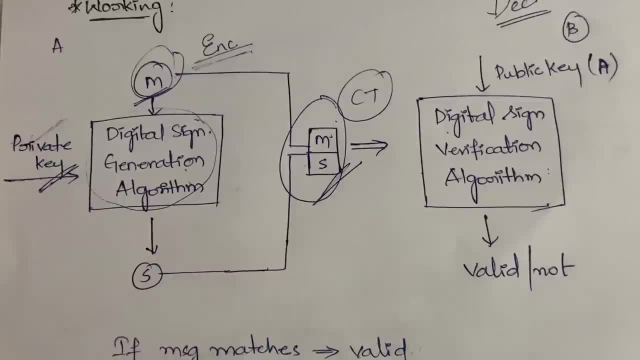 have personal experience in bank. when I signed, they call me and ask whether it's your signature or not, because the strokes were a bit different. right in my 10th grade I was forced to. you know, my teachers and everybody said that I have to write my full name as a signature and from then I'm continuing the same and in 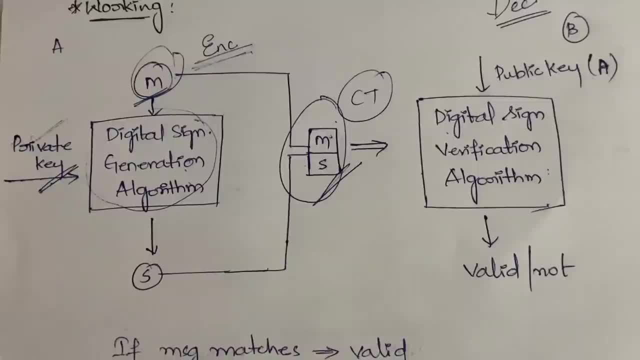 order to write my full name as a signature. sometimes, obviously, strokes go different, right? so if I sign hundred times, hundred times different sign, only I'll do so. that is so, even if small strokes are different. also, even you know underlines or whatever it is. so it will not consider so by if the message is: 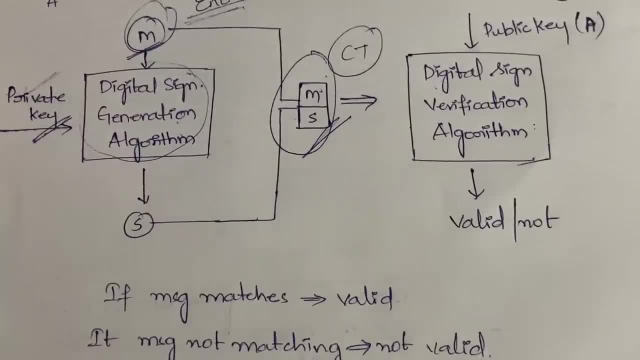 matching, you can say valid. if the message is not matching, you can say that the digital signature which has been did is not valid. got it. so this is about the digital signature. I hope this video is clear for you if you hit the like button and also share it with your friends and family, and I will see you in the next video. bye, bye. 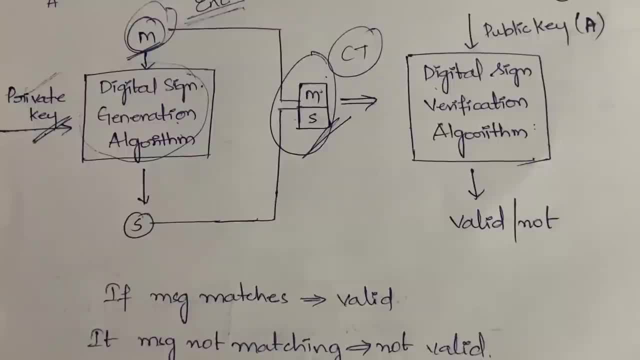 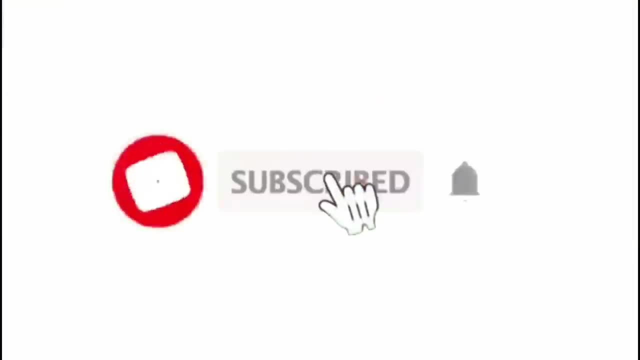 with your friends and if you still having any doubts apart from what I've explained this video, just let me know in the comment section. I'll be very happy to answer your questions. and thanks for watching the video till the end. let's meet up soon the next coming video with another topic.